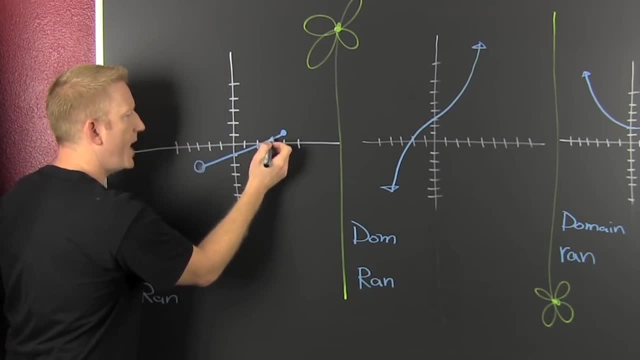 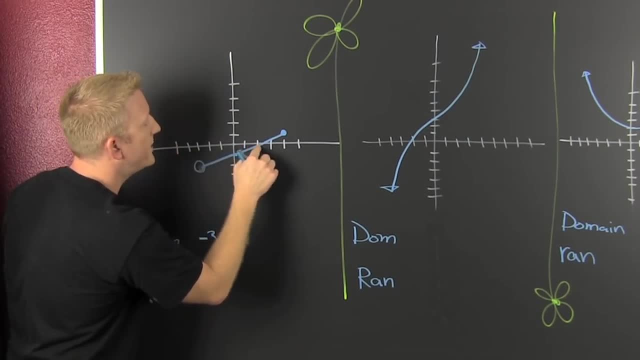 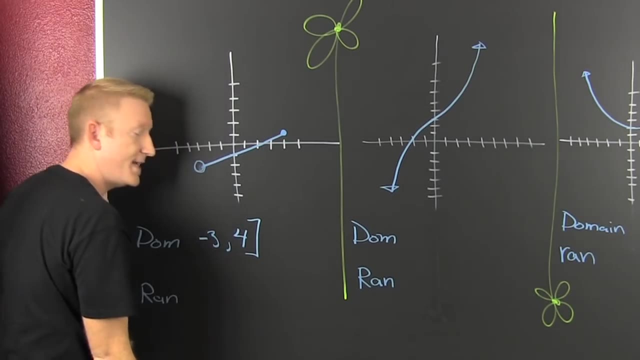 It appears to be a minus 3 all the way to 1,, 2,, 3,, 4 in the positive. Now that's a closed dot, so that is represented and I'll represent it like that. but this side is an. 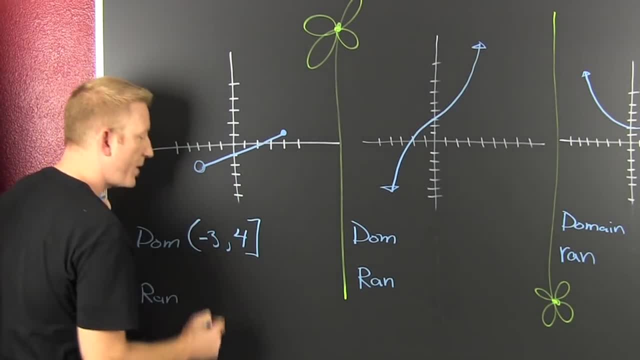 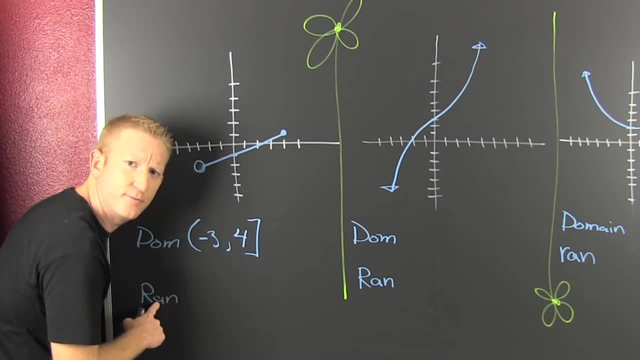 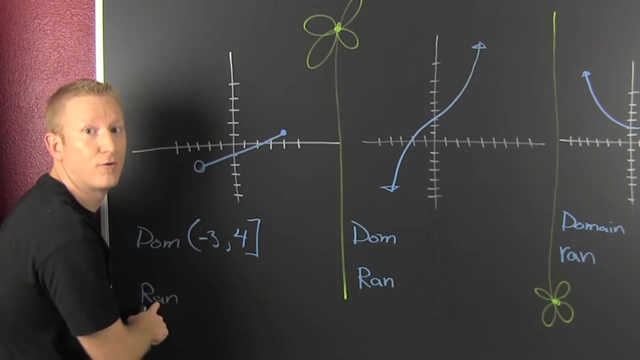 open dot, so it's represented by open and you're left with that Klopin interval, half open, half closed. and then I ran down here to the range. She liked the boy with the big old chain. I ran down in the big old range. Okay, it's not that one. You didn't like that, How'd. 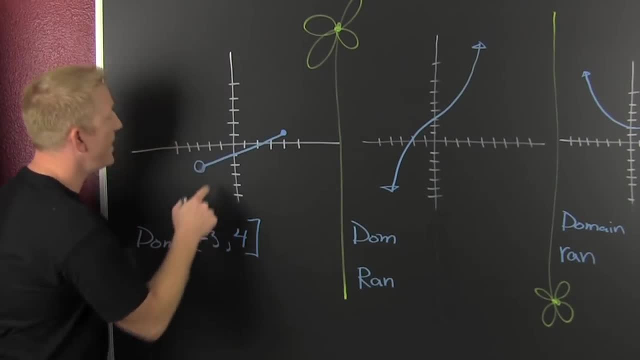 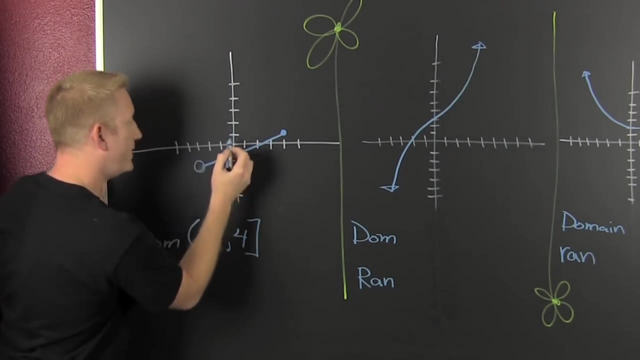 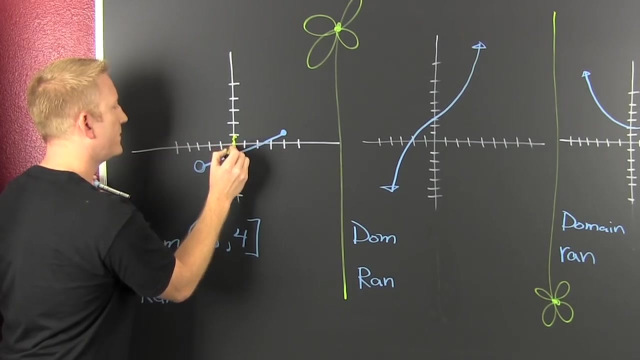 you like that? Okay, so then the range is the set of all y values and that's why my range goes from a minus 2 to 1, because when I'm looking at the range, I'm looking at this stuff, this stuff, this stuff, and stop, because it's the set of all y values and that's why. 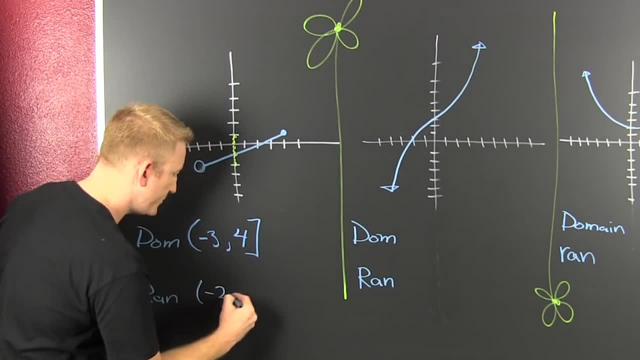 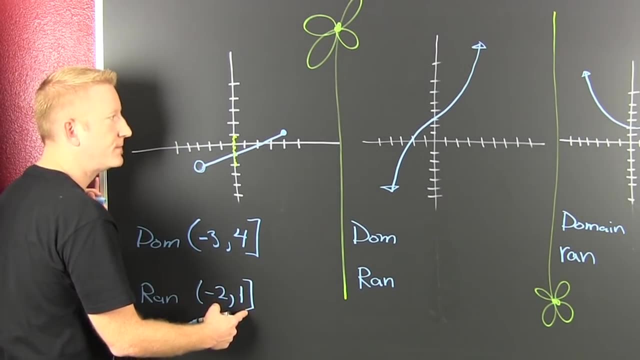 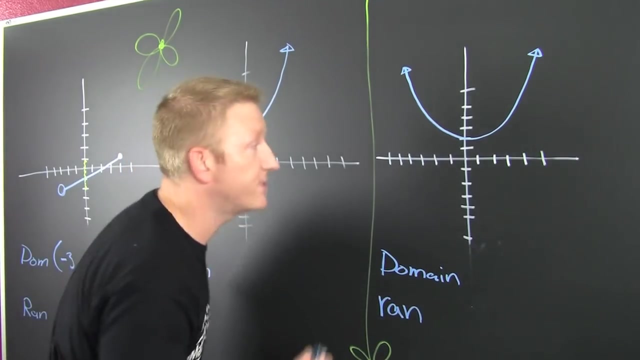 I go from 1. minus 2. 2. 1. Fun, Open on this side, closed on that side. Now I side and we're, with this example, over here. Okay, You ready. The domain is the set of all x values. Which x's are represented. Oh, 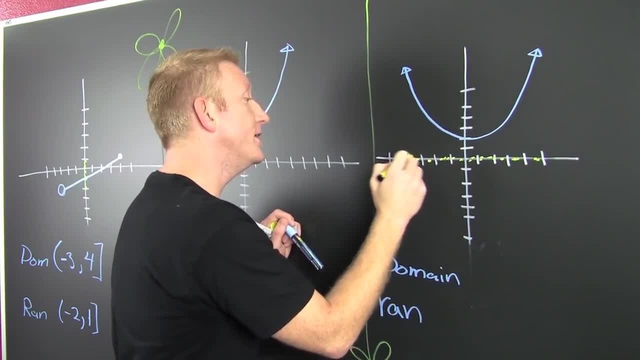 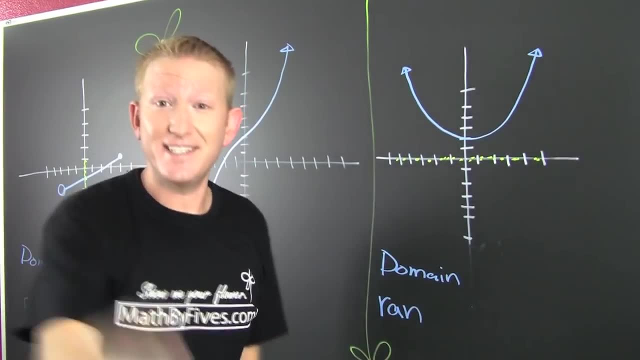 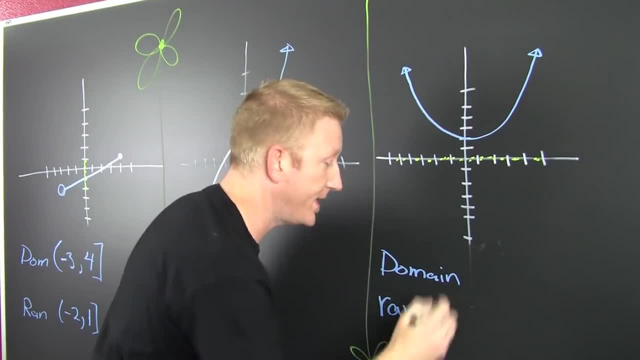 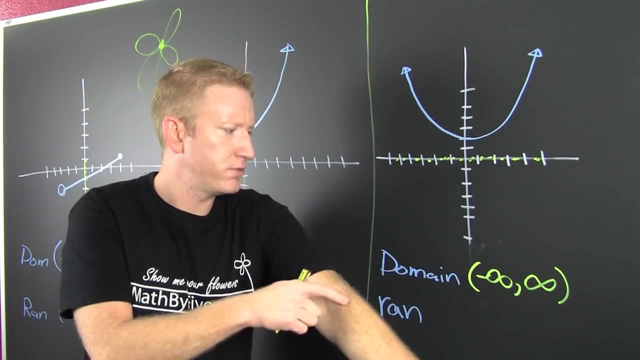 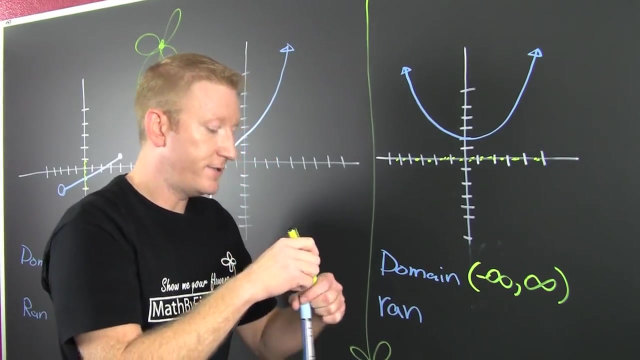 It just continues to go. so all of the x values are represented, and that's how I represent my domain, from minus infinity all the way up to a positive infinity and beyond. Let's buzz on down to the range. Sure, The range is the set of all y values, Is this? 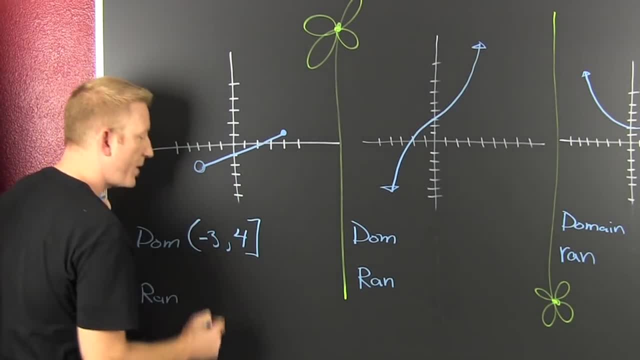 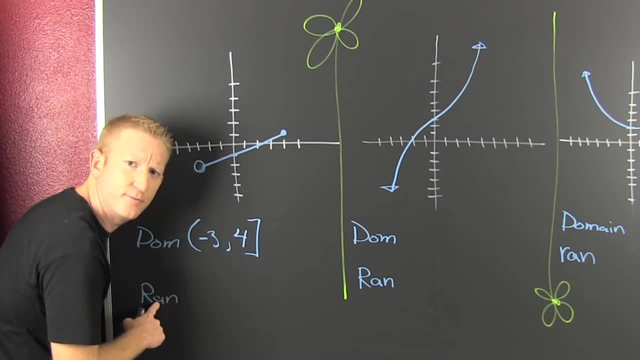 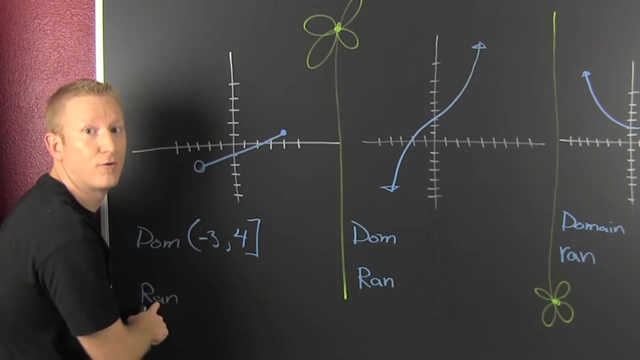 open dot, so it's represented by open and you're left with that Klopin interval, half open, half closed. and then I ran down here to the range. She liked the boy with the big old chain. I ran down in the big old range. Okay, it's not that one. You didn't like that, How'd. 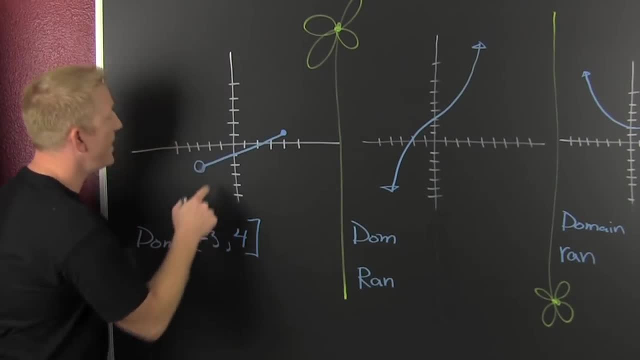 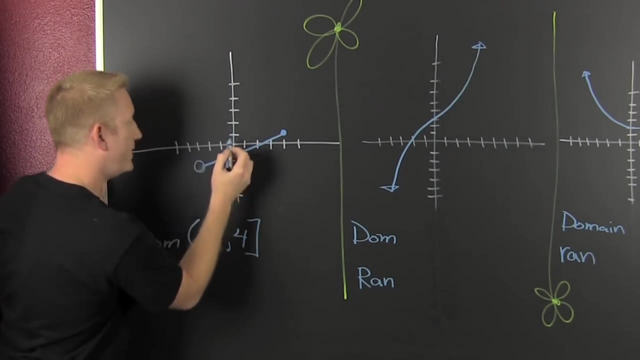 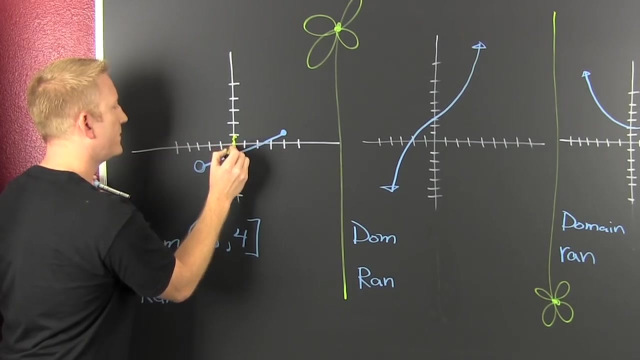 you like that? Okay, so then the range is the set of all y values and that's why my range goes from a minus 2 to 1, because when I'm looking at the range, I'm looking at this stuff, this stuff, this stuff, and stop, because it's the set of all y values and that's why. 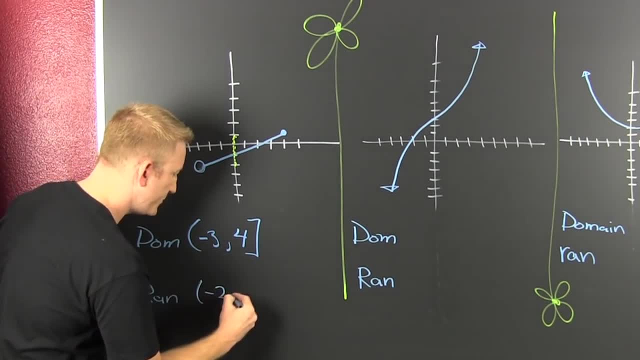 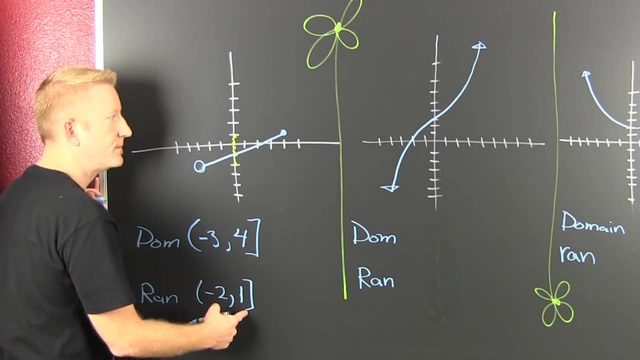 I go from 1. minus 2. 2. 1. Fun, Open on this side, closed on that side. Now I side and we're, with this example, over here. Okay, You ready. The domain is the. 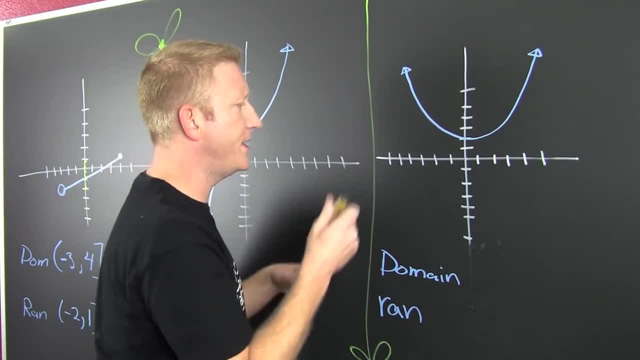 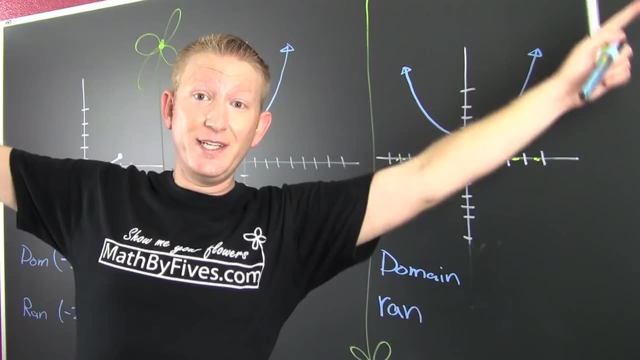 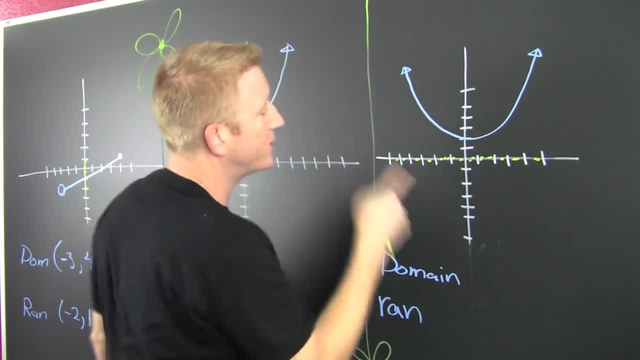 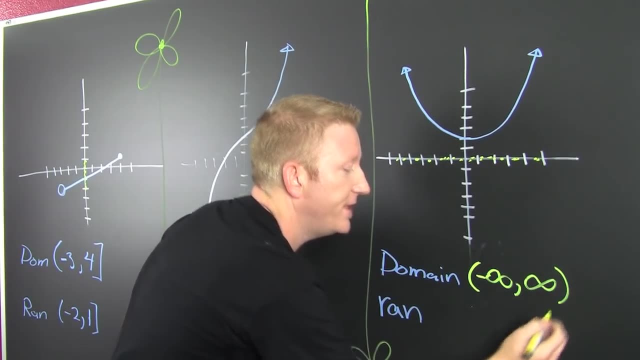 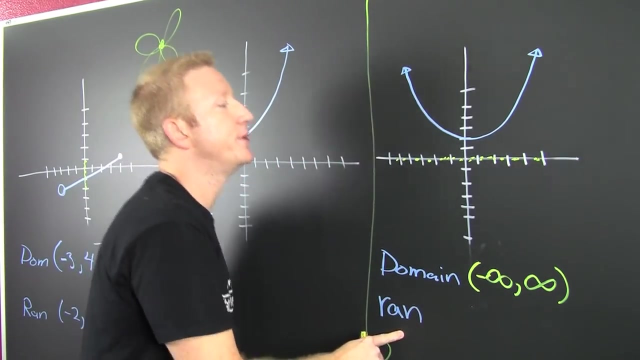 Just It doesn't stop, It just continues to go. so all of the x values are represented, and that's how I represent my domain, from minus infinity all the way up to a positive infinity and beyond. Let's buzz on down to the range. Sure, The range is the set of all y values, Is this? 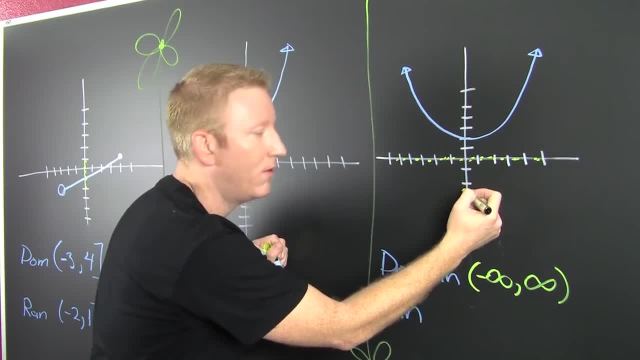 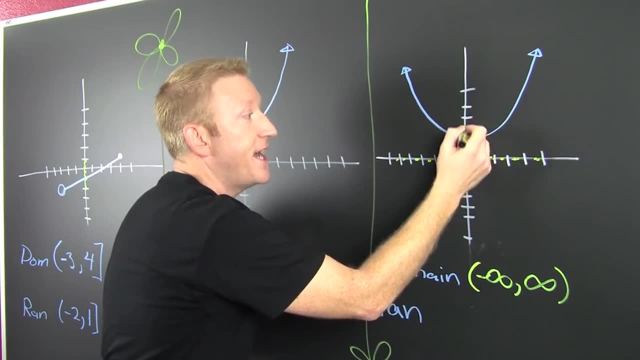 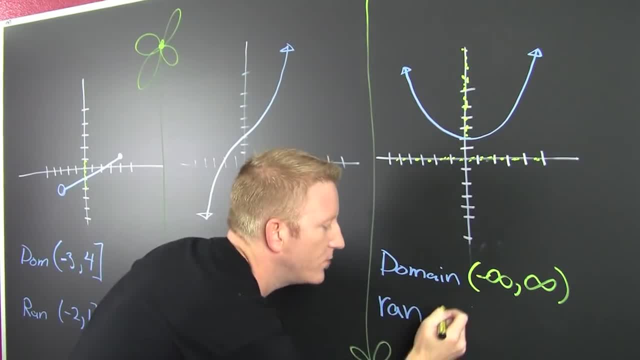 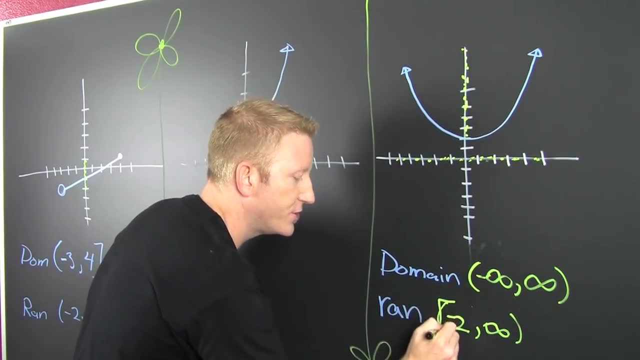 Our range is restricted to everything above 2.. So then we do go from 2 to infinity and beyond. Do I include the 2?? Sure, Because it's included in the range. Now I ponder and I wonder: Does the order matter? Yes, This is interval notation Lowest.